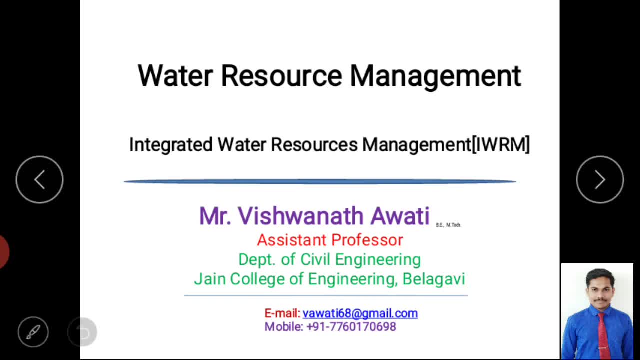 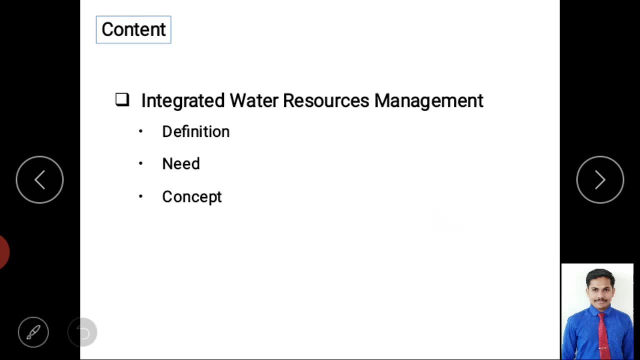 is integrated water resource management. It is a recent topic and recent method of water resource management. and myself, Vishwanath Avati, assistant professor in a department of civil engineering, Jain College of Engineering, Balagavi. So now we will see what is the main discussion of today's. 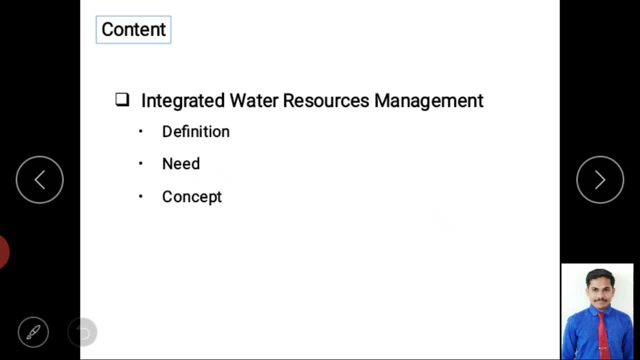 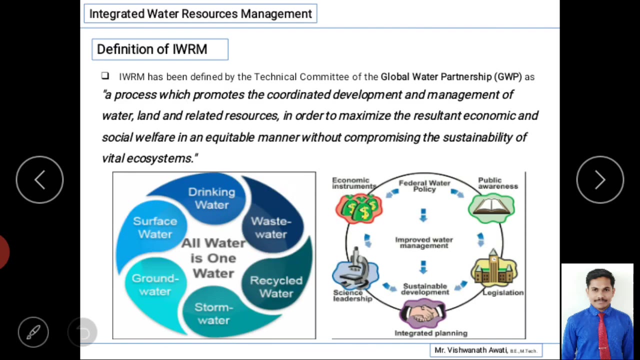 video. So in this video we are mainly discussing about definition of integrated water resource management: need of integrated water resource management, then concept of integrated water resource management. Now we will understand what definition of integrated water resource management. So here it is. according to global water partnership right, and they given a definition. The definition: 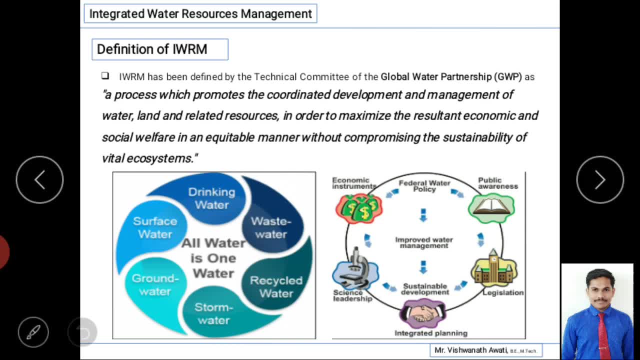 is. it is a process which promotes the coordinated development. So they are telling that it is a coordinated development among the different stakeholders and management of water, land related resource. So here we are not focusing, here they are not focusing only water, even though it is a water related, but when we are focusing on land and related resources, So here we are. 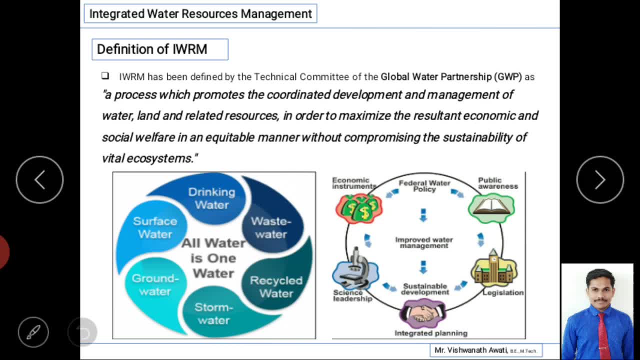 trying to conclude the picture. Okay, so here, air is a water, land related resource in order to maximize resultant economy, resultant economic, economic means: what benefits? right, You want to benefit us with the some benefits and social welfare. you're getting economic benefits as. 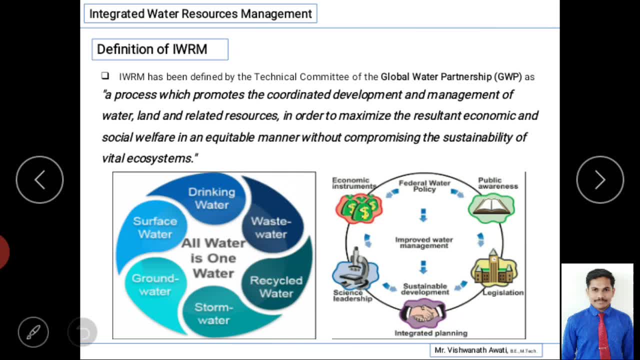 well as society improvement, social welfare in an equitable manner. even we're maintaining equitable manner without compromising the sustainability of vital ecosystem. e aqui temos que concentrar прежде. all here we have to focus. one is: it is a quarter, so coordinated among the planner, user, policy, maker of management, and, and it is 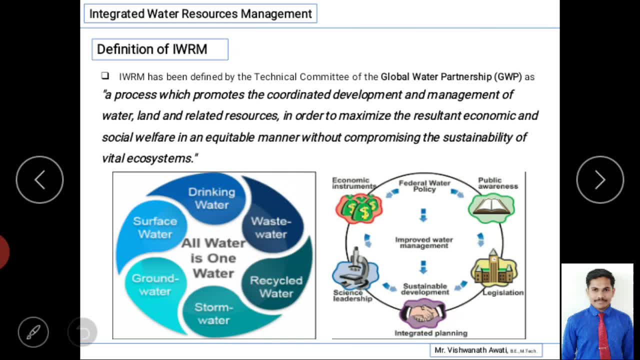 a management of water as well as water related resources- one is land and one is biodiversity- in order to maximize the resultant economy means a small investment, more profit of, and as well as social welfare in an equitable manner, without compromising the ecosystem. even we are not neglecting the ecosystem. 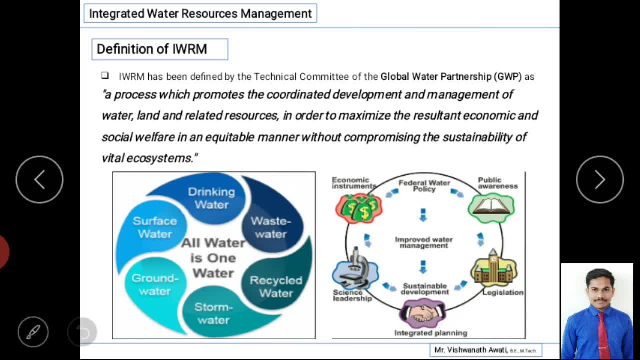 for example, how it is called as the integrated, because when we are going for water resource management we have a different type of water. one is drinking water. so when you supply for drinking water, obviously at the end it will make a waste water, and even after the waste water if you are making recycling, even 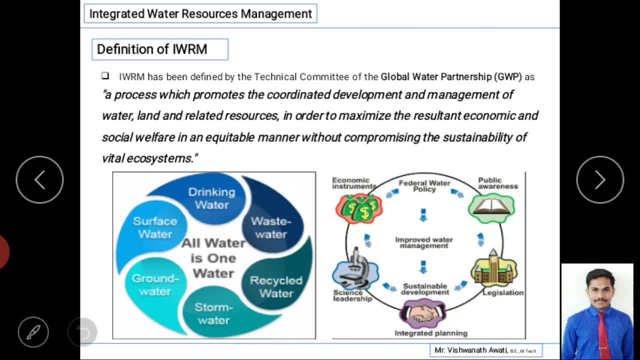 our recycled water right. so then, strong water, ground water, surface water- these are all three types of water which is available on the earth. so whenever we are making the planning, we have to take the considerations of all three means. all three are all are interrelated, and even when you go for management of 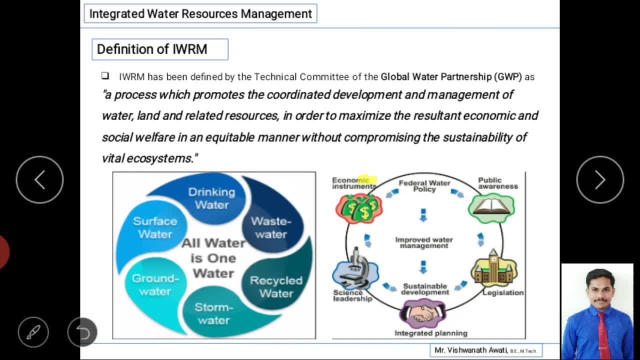 this we have to consider the economy means. you know, even economics is very important, like investment and profit. so then public awareness, even people has to know about it how to is, and if people are don't know, then entirely the system will fail. so even we have to make some rules and regulations then integrated. 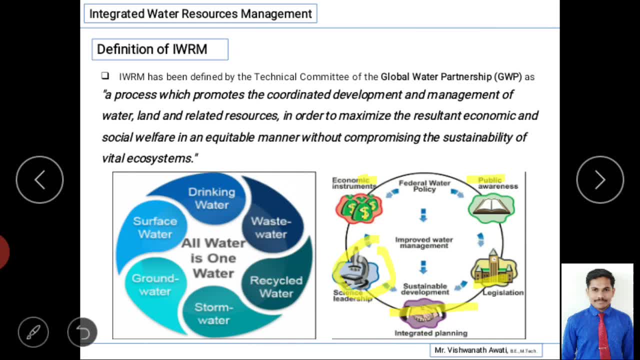 planning and even we have to go for scientific analysis. whatever management we are taking, that will be based on the scientific and based on the research and it improves the water management right. sustainable development: we need developmental activities, but without compromising the ecosystem. so environment is very important. I cannot deal with the environment right, right it. 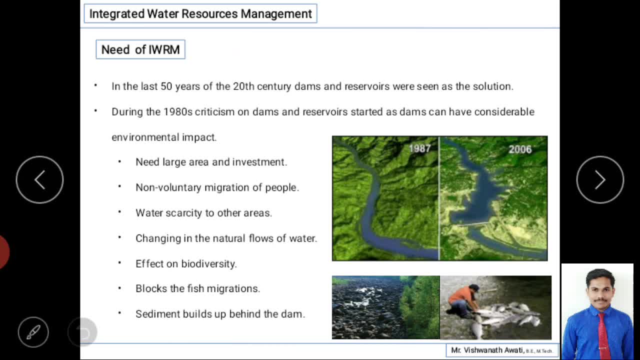 is a definition. now we will see why actually needed. why integrated water service management? already we are making the water resource management. but why you required? because in, like you know, 50, 50 year in, as of now it is a decent topic, but earlier we have water resource. 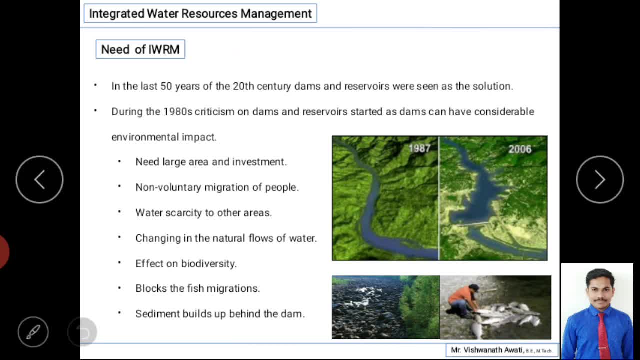 management based on the construction of dam. we thought that dam will give all the solutions of water resource management but recent, recent, recent studies they are telling that dam has some impacts on the water resource management. it has an impact on environment. so impacts like need, need a large area and investment. it required large area. right, because he has to store the tmc. 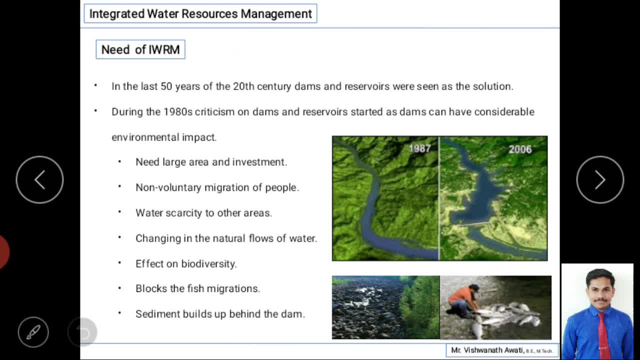 of water means it required large area. so when large area is required means already some areas will be used for agriculture, area will be used for forest, area will be used for settlement. so when we are planning the dam, then we have to make the migration of the species as well as the people. 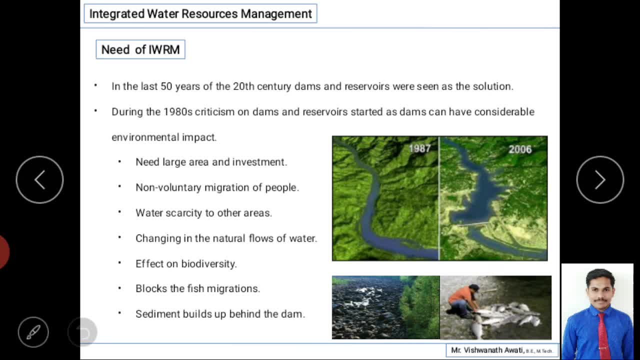 so that's what? non-voluntary migration of people, right? so then, when you are construct, when we are constructing the dam, water will be stored on upstream. so what about the dam stream? even it makes the flooding on the upstream and it creates the water scarcity in a downstream. then changing. 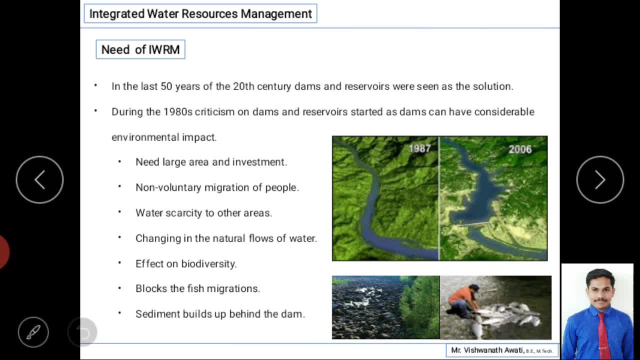 the natural flow of water effect on the biodiversity. effect on the biodiversity means what we require: the huge construction activities. when we require the huge construction activities means we have to create the road. so when we have to create the road, means we have to make the removing of plants means for deforestation. so, due to the deforestation, 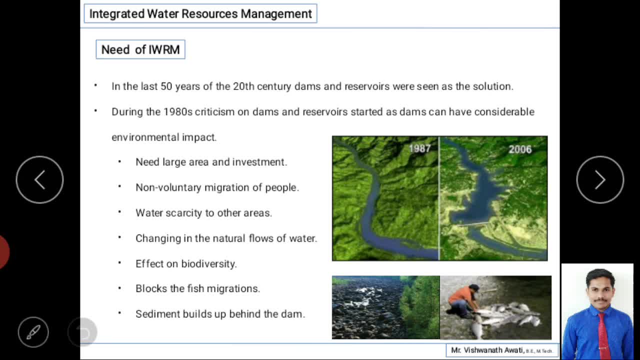 many like species, or birds or some many insects. they will lost their livelihood. so that's what it will impact on the biodiversity. then some species will be there, some species like a fish- they are migratory fish- right based on the climatic condition, based on the temperature, based on the 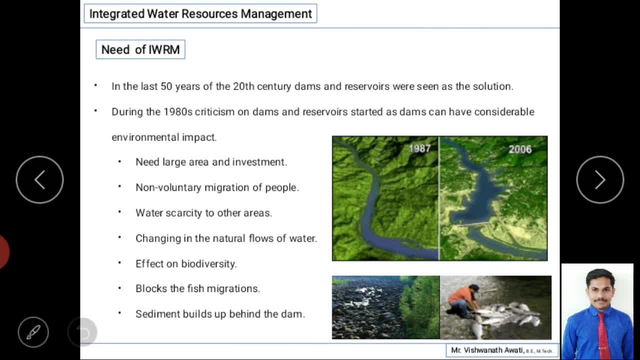 climatic condition, they will migrate from one place to another place. so when there is no barrier then they can move from easily from one place to another place. when we are creating barrier like a dam, so then it affects on the migration. finally it causes the death of the fish, then sedimentation. 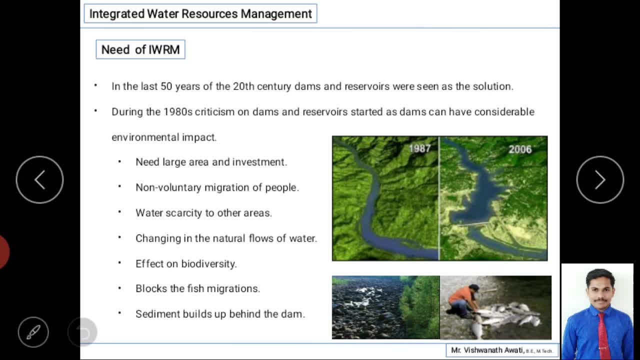 at the dam. so even it caused that sedimentation and even sedimentation will be lost at the downstream and it may cause quick releasing of water. it may cause the erosion right, quick erosion. these are the some problems due to the construction activity of dam, but these are the 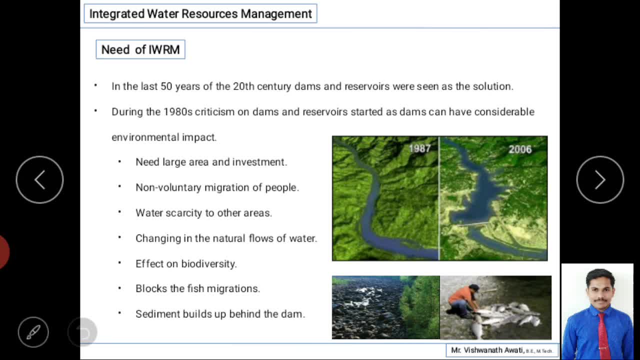 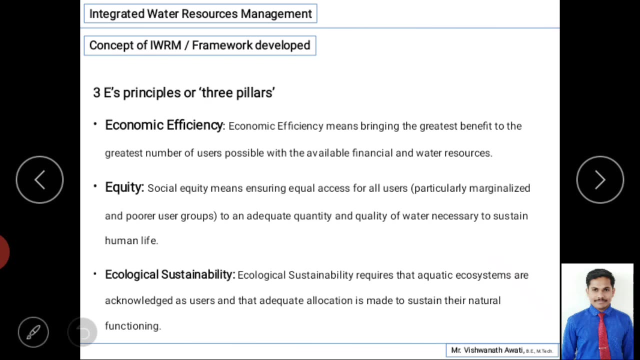 impacts we can overcome with the help of integrated water source management. so we'll see how we are overcoming the these problems right one by one. so now we will understand concept of integrated water source management. what actually integrated water source management on what it depends. so actually, framework developed means they want to do what actually it has to be work on. 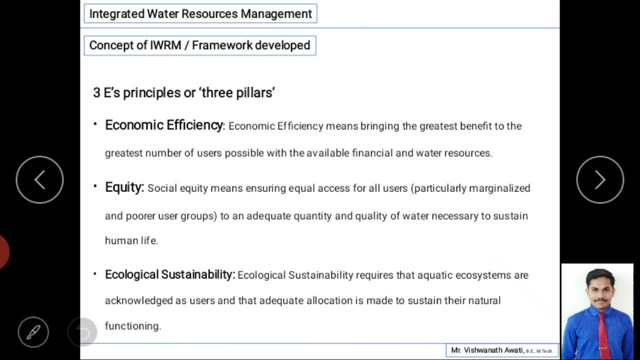 the main three principles. so one principle is, or even it is called as a 3e or three pillars of integrated water resource management. so one is economic efficiency. economic efficiency means what, like we have to think about our investment or our recovery, so your small investment has to be made, but more benefit will be taken from that and that benefit. 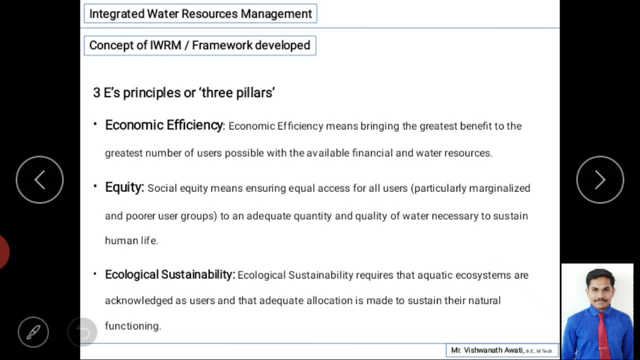 has to be created for all, not for only one species or only for human. even that investment and efficiency has to create a good Society as well as ecosystem around that right. so that is what economic efficiency greatest benefit to the number of users, greatest benefit to the greatest number of users. so here, number of users are. 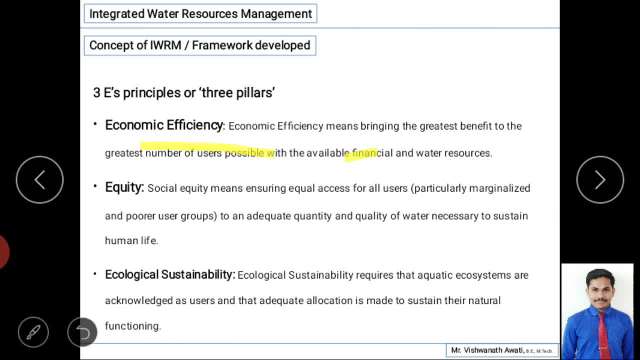 creating more then with the available finance and water resource right. so next one is equity. so it is not a market equity, it is like no equity among the social condition. social equity right ensuring the equal access to all the users. here we are, what we are making. we are making the 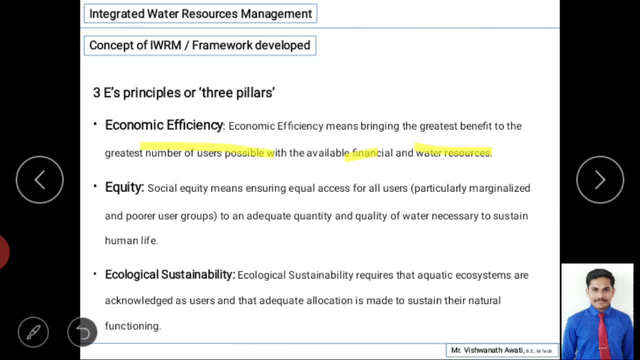 accessible to all the type of people, all the type of people like poor people, rich people, marginalized people. but mainly we are taking considerations of poor people and marginalized people and they has to get a good quantity of water as well as good quality of water, which they require for sustainable life or good life, right? so even here quality is taken considerations. 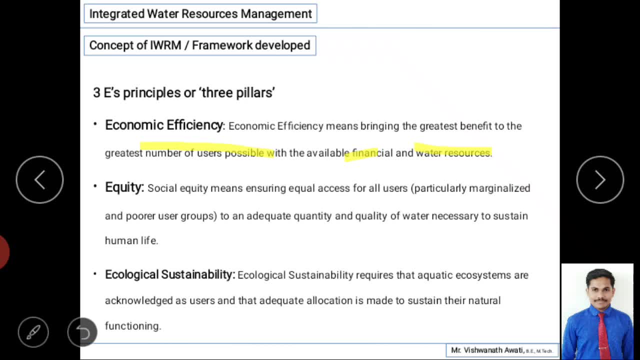 even sufficient quantity of water also has taken the considerations and it is what i told. it is a human relationship related activities, but even here considerations of environment is also considered. even it is given a more important you can see- ecological sustainability. in the ecological sustainability mainly we are taking considerations of how much water is required and adequate allocation. here 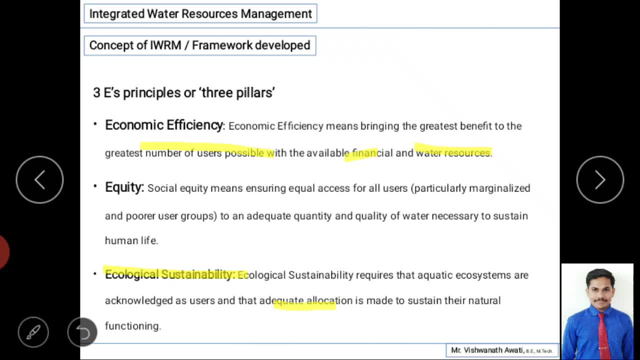 adequate allocation to the natural right. nature is there and even nature for nature. it has some functioning activities, means even plant growth will be there, photosynthesis activity will be there, right, right, right, and grass development. all the functions will be there of environment and for that, how much water. 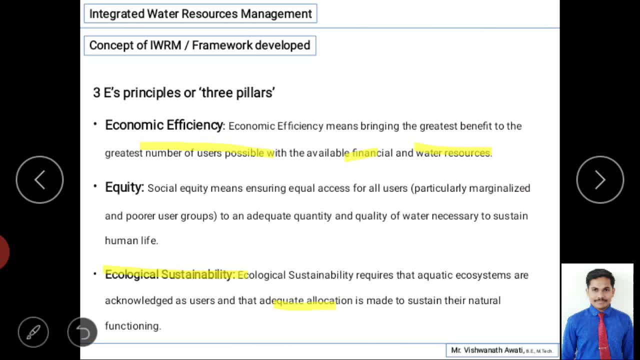 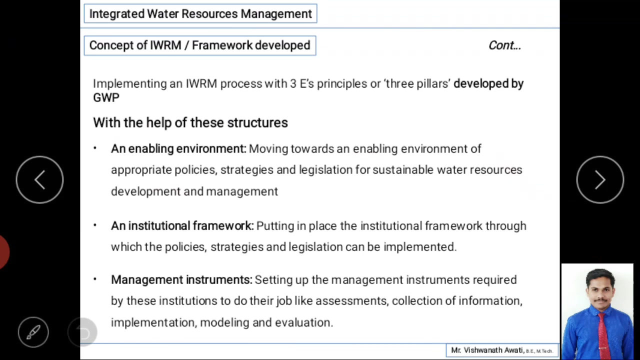 is required that much of water is given consideration to the ecosystem. right here, ecosystem is taken considerations and accessible to the all the people, and even it is taken a considerations of economy, investment and greatest benefit. to achieve this we require some structure. we required structure and here these structures are mainly one is enabling environment. 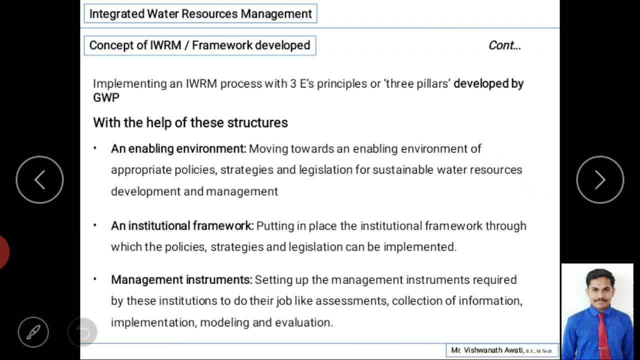 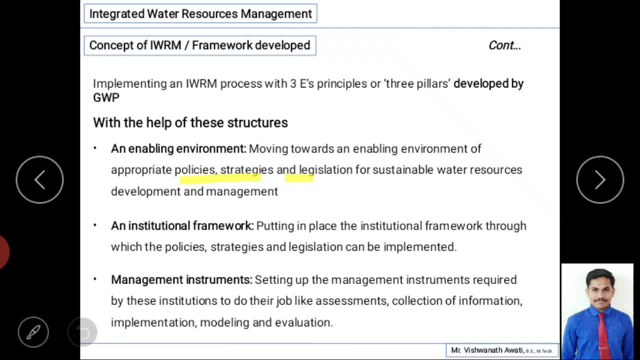 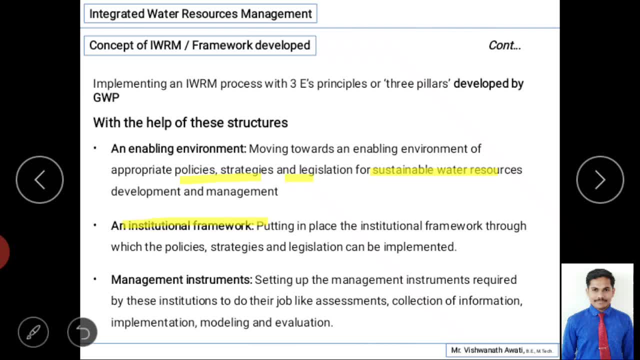 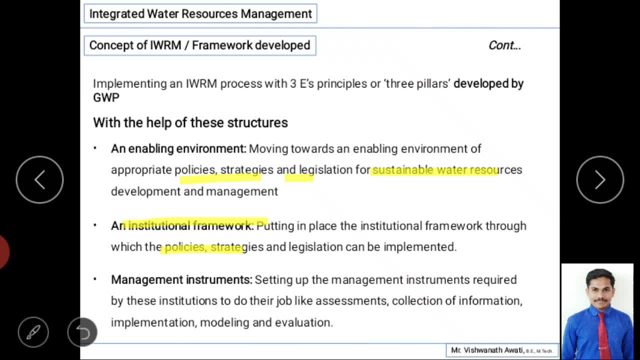 means we have to tell duties of all the persons they has to do under the law and rules, right. so that is what institute. so then we have to provide the basic facilities to carry out all the activities. that is what management instrument. management instrument means whatever activities are there. 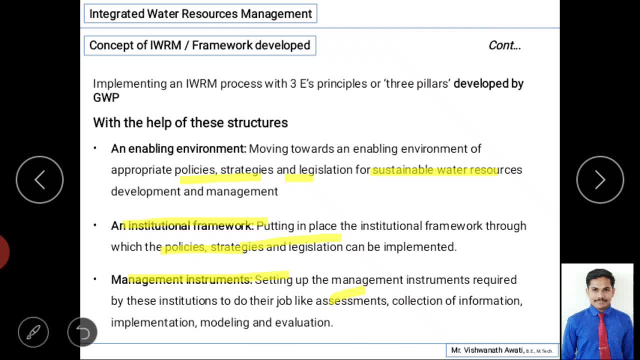 like assessment right. whatever you want to take, any activities there has to be, as a made. assessment means we have to go for all the scientific analysis, to do the scientific analysis and collection, collection of information, implementation, right, modeling and evaluation. so many activities will be there. it means that to complete enabling environment and institute and to make it successful. 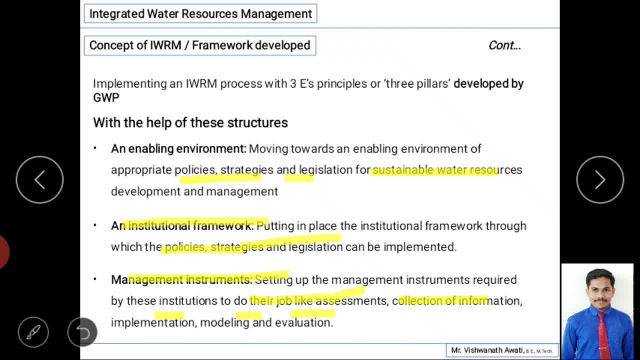 they has to do some jobs, so the jobs will be given and some capacity development or some whatever resource are required to carry out all this activity has to be provided under management management instruments, management instruments- right, so these are the three main structures to achieve the basic principle of three e's. so now we'll see how they are principles, and 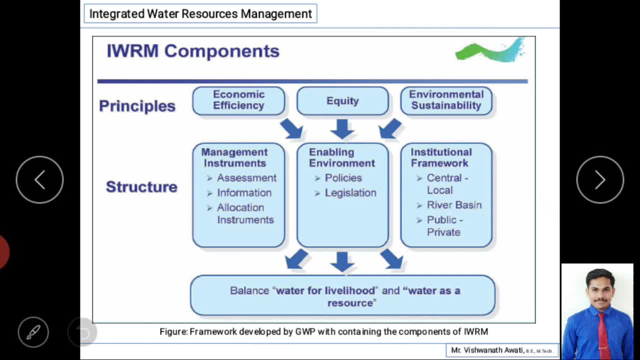 structures interrelated, how it is interrelated and this entire analysis is also called as integrated auto resource management components. integrated auto resource management components, right, so here it is composed of principles, then it is composed of structures, then based on that result, so you can call this is a result of these two. so one is principles, so here principles are. 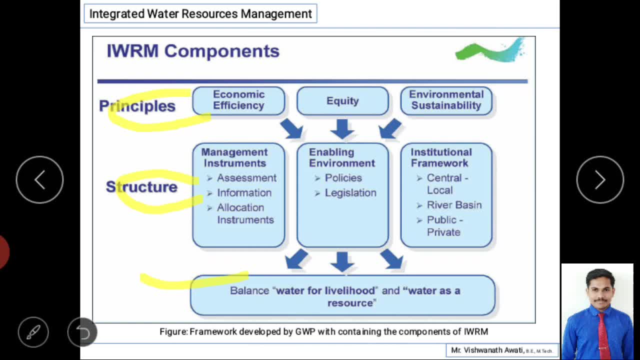 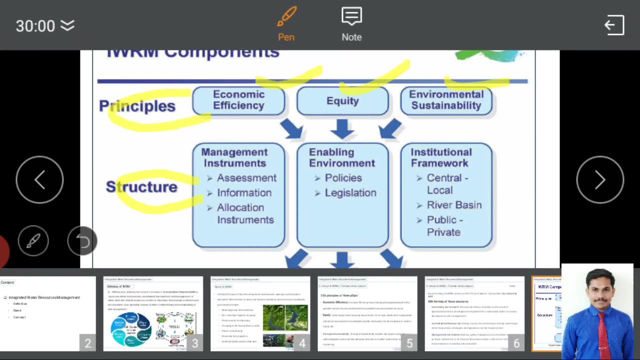 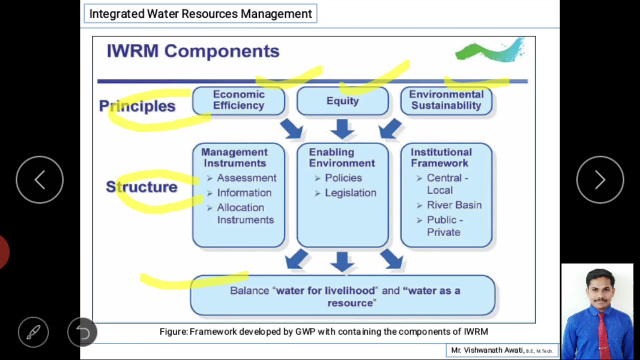 divided into three e's, again right, as i explained earlier: economic efficiency, equity and environmental sustainability. environmental sustainability- here considerations of economy is also taken. then equity and environmental sustainability, then how to achieve this? with the help of structure. so structure is also here: management instruments right. assessment, information, allocation instruments, right. so then, 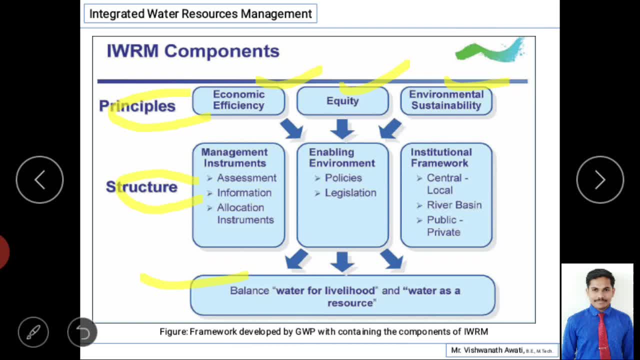 enabling environment. so how to enabling environment means maintaining in a good condition. so how to maintain in a good conditions by rules and regulations like water act, air act, right forest act, fishery act. so many acts will be there and rules and regulations will be there. based on that, we are making the good environment. then how to maintain this good environment? we are.